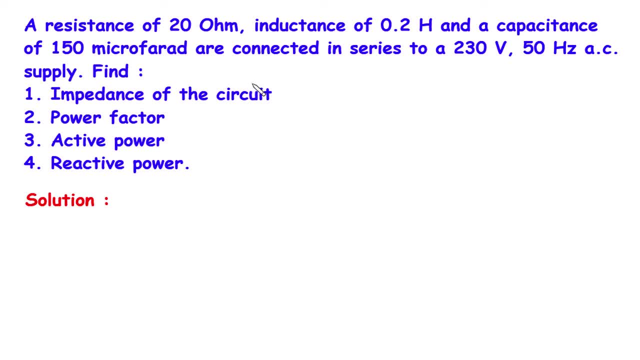 If you find this video helpful, then feel free to donate whatever amount you can. link is in the description below: A resistance of 20 Ohm, inductance of 0.2 Henry and a capacitance of 150 microfarad. 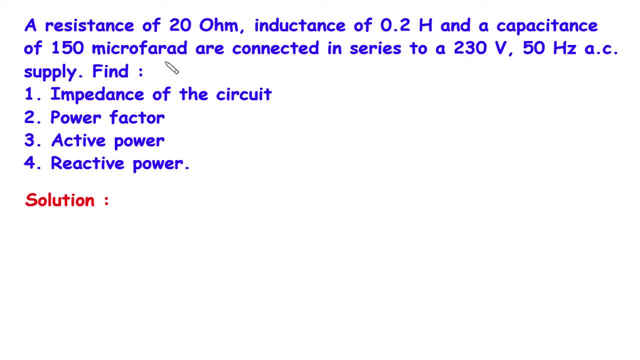 are connected in series to a 230V 50Hz AC supply. Find: 1. Impedance of the circuit, 2. Power factor, 3. Active power and 4. Reactive power Solution. First of all, we will write what is given. 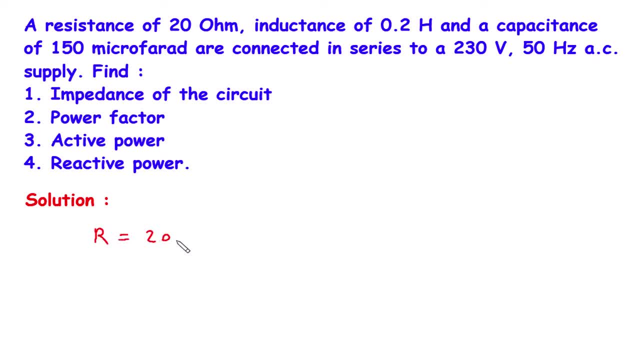 The value of resistance is given, so R is equal to 20 Ohm. The value of inductance is given, so L is equal to 0.2 Henry. The value of capacitance is also given, C is equal to 150. microfarad are connected in. 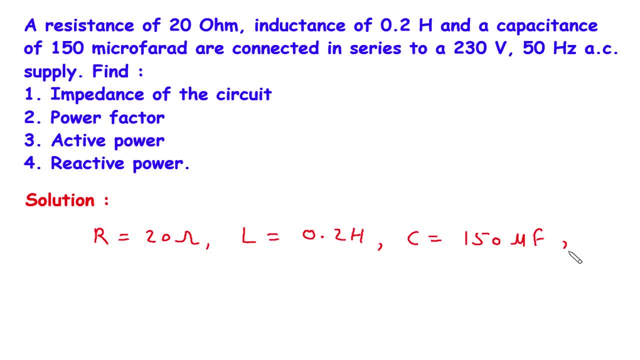 series to a 230V. The value of voltage is given. voltage V is equal to 230V. The value of frequency is also given. F is equal to 50 Hertz. Now we have to find impedance of the circuit. 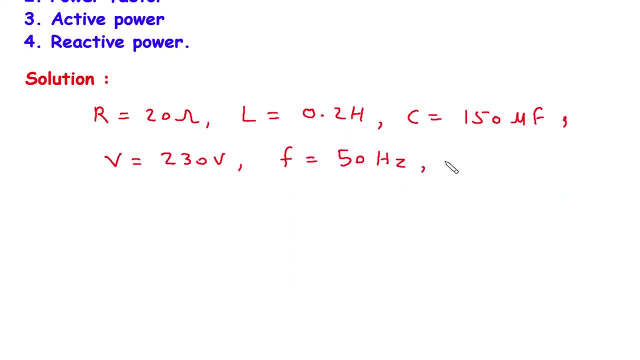 So impedance of the circuit we have to find that is Z. So first of all we will directly write the formula: Z is equal to under root of 0.5. V. It is always like this: Pay your time, I am going to write it as 4 into 3 instead of 4 into 3.. 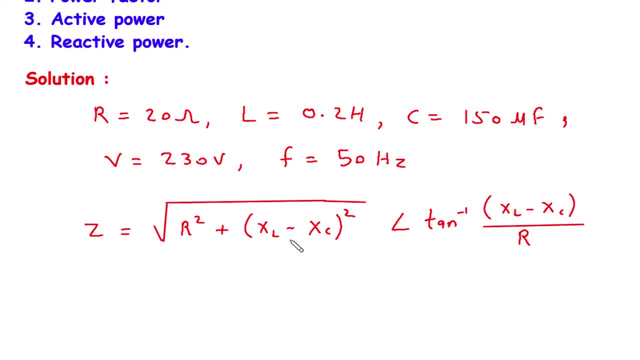 Thank you, Bye, bye, this R, but we don't have the value of XL and XC, So first we will find XL, calculate XL, that is, inductive reactors. the formula is 2 pi, FL. So we will substitute all the values: 2 pi multiplied by frequencies- 50 Hertz- multiplied by L, is inductance and its value is 0.2 Henry. 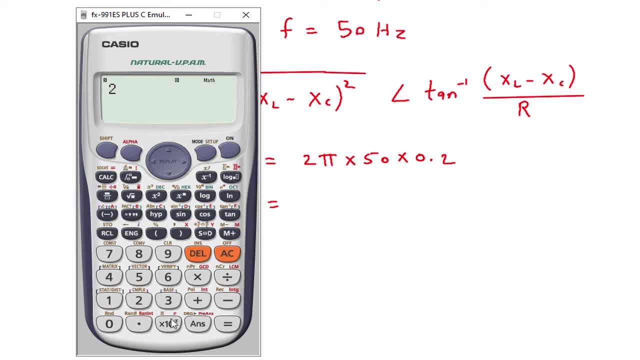 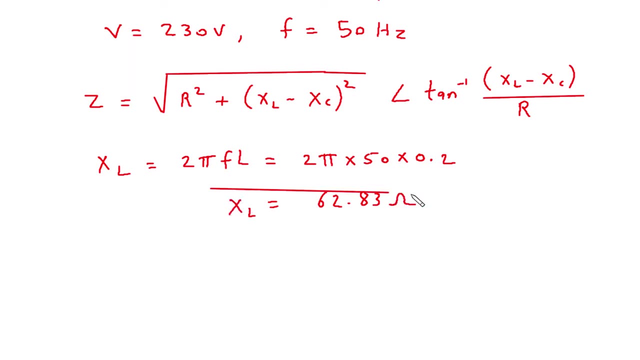 So this will be 2 pi multiplied by 50, multiplied by 0.2.. So it is 62.83, 62.83 and its unit is a home. This is the value of XL. Then next we have to find XC. to calculate XC, there is: 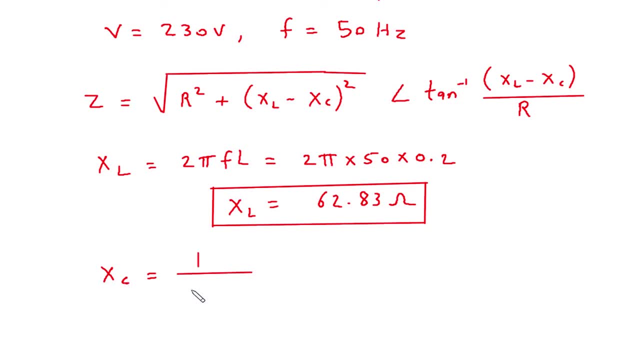 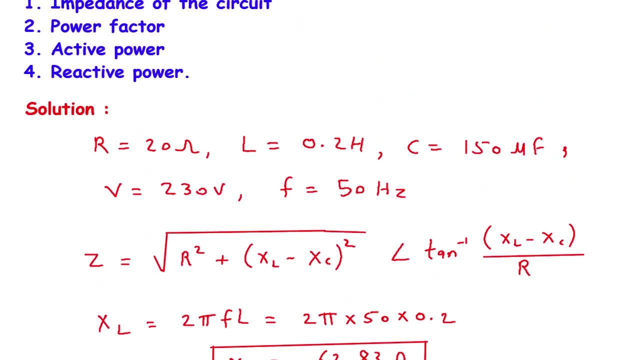 a formula: XC is equal to 1 upon 2 pi F, XC, 1 upon 2 pi F, XC, c. So this will be 1 upon 2 pi. frequency value is again 50 multiplied by c. c is capacitance. 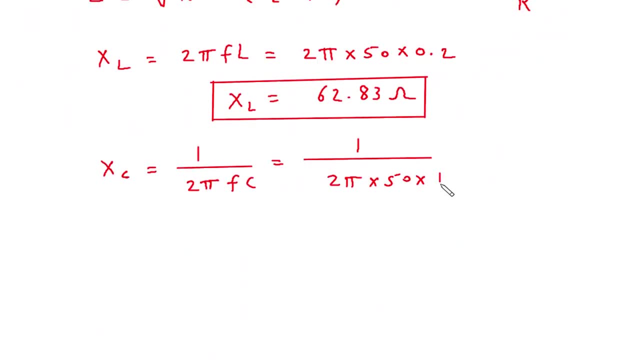 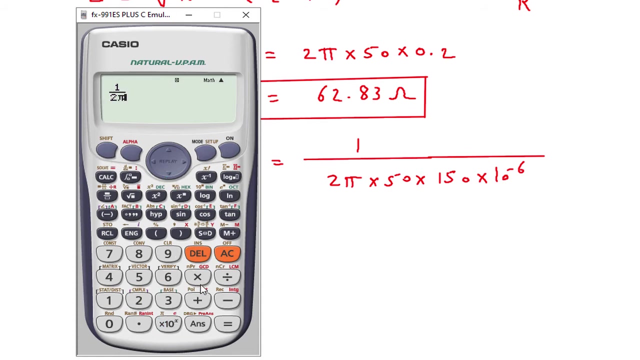 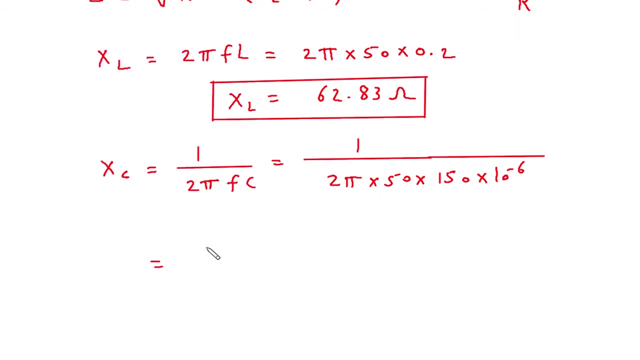 and it is equal to 150 microfarad. So this will be 150 multiplied by 10 to the power minus 6.. Now, if we solve it, so this will be 1 upon 2 pi, multiplied by 50, multiplied by 150, multiplied by 10 to the power minus 6.. So it is 21.22,, 21.22, this is the value. 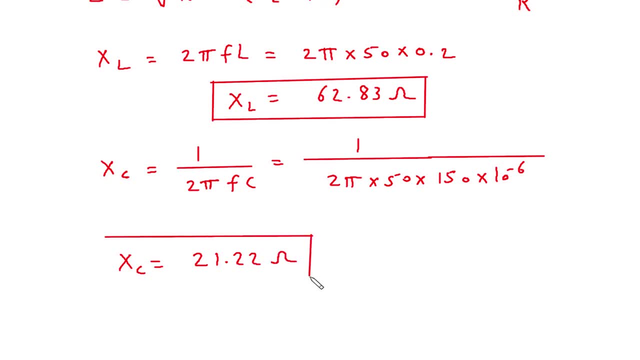 of xc and its unit will be 0. So we have xc and then by Ky- which means the unit will be 0.32.. So this just konkretized. Now we have the value of xl and xc. so we will find first of all xl minus xc, so xl minus. 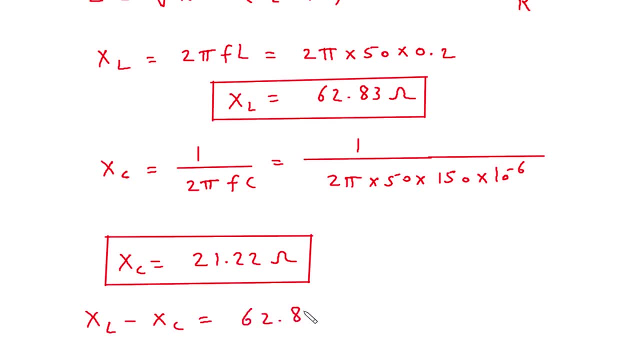 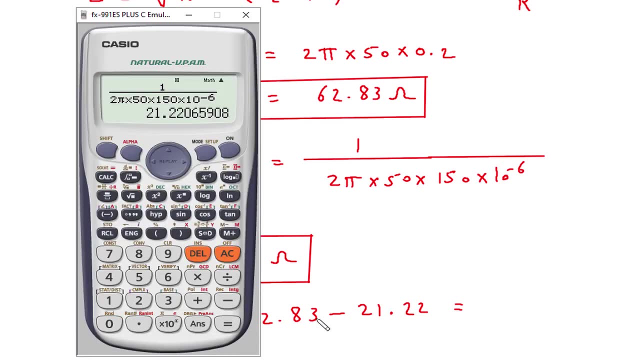 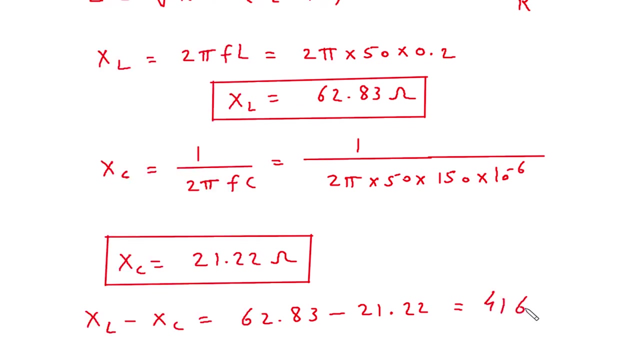 xc will be 62.83 minus 21.22. so this will be 62.83 minus 21.22. it is 41.61, 41.61 ohm. Now we will find xl minus xc. so we will find where is the value of xc. 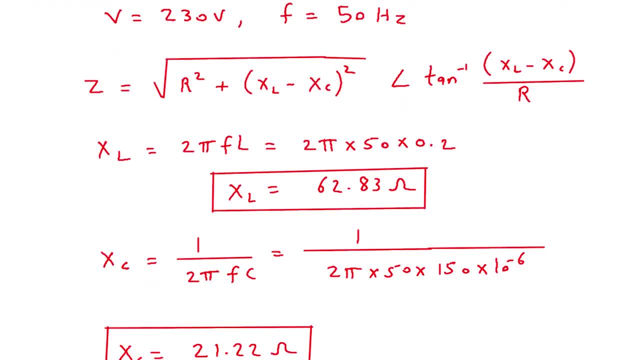 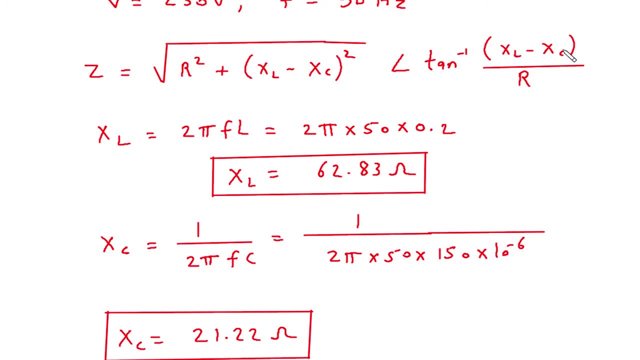 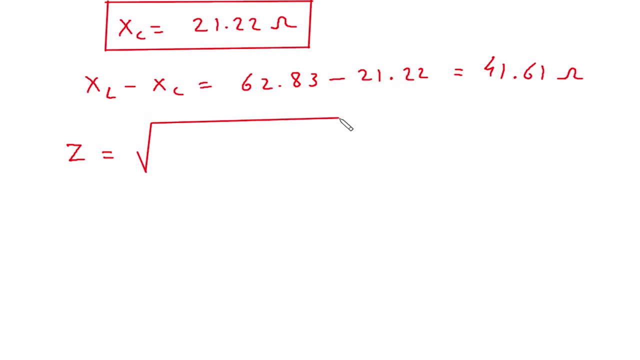 Now we have to find impedance Z and its formula is: R square plus XL minus XE, whole square at an angle of 10, inverse of XL minus XE divided by R. So we will substitute all the values. Z is equal to under root of R. The value of R is 20 ohm. the resistance value is 20 ohm. 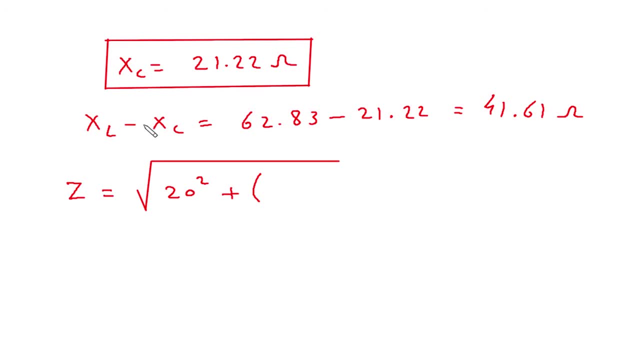 its square plus XL minus XE whole square. So XL minus XE is 41.61, whole square at an angle of 10, inverse of XL minus XE. So XL minus XE is again 41.61 divided by R. The 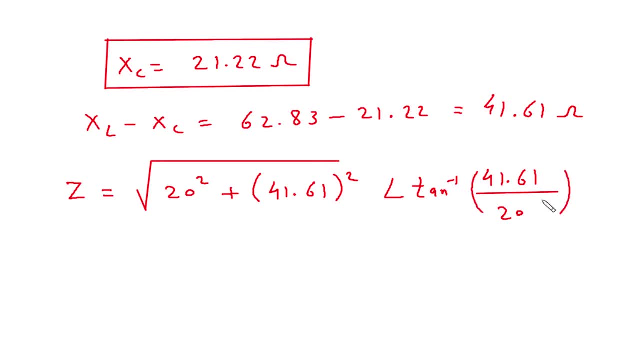 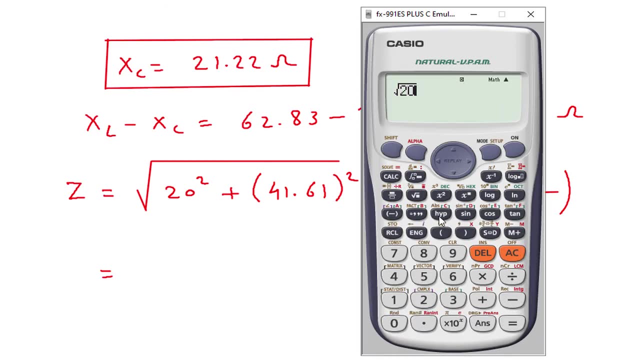 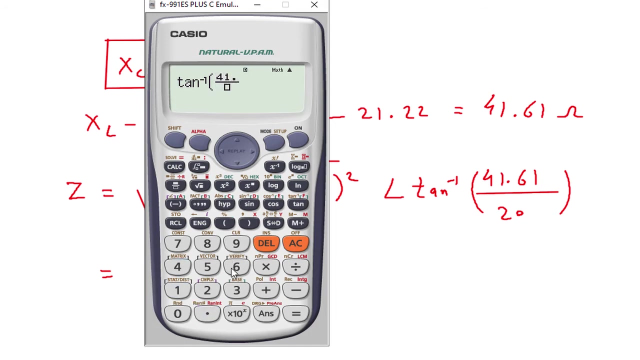 value of R is 20.. Now if we solve this, so we get under root of 20 square plus 41.61 square, It is 46.16.. 46.16 at an angle of 10, inverse of 41.61 divided by 20.. So it is 64.32.. 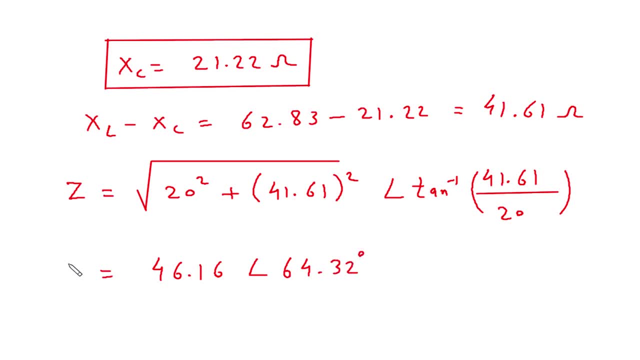 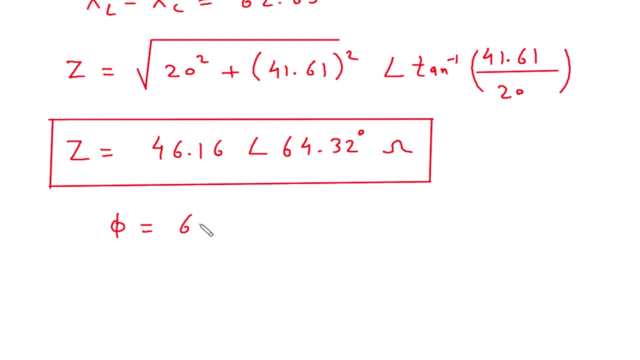 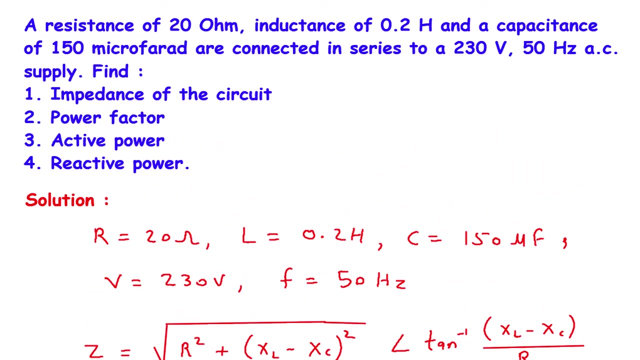 Now, since it is impedance, so its unit will be ohm. So this is the answer for impedance. Then, from this impedance, we have also found the value of angle phi, and it is equal to 64.32 degree. What we have to find next? We have to find power factor. So power factor. 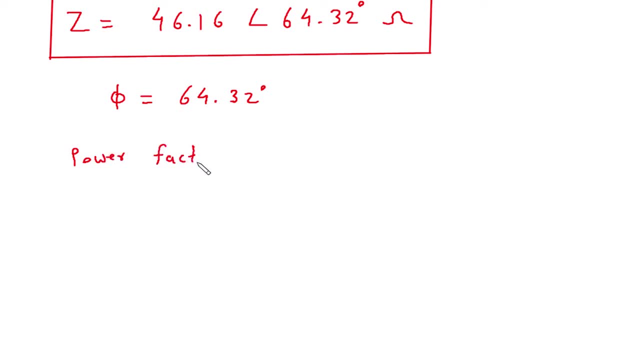 is equal to. Power factor is equal to 64.32.. Power factor is equal to 64.32.. Power factor is equal to 64.32.. Don't think that the value of power factor is equal to 24.. So power factor is equal to. 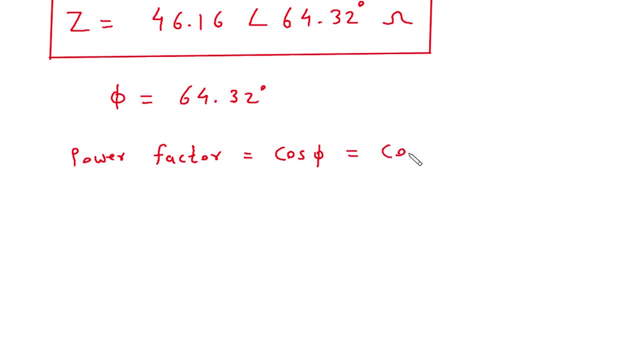 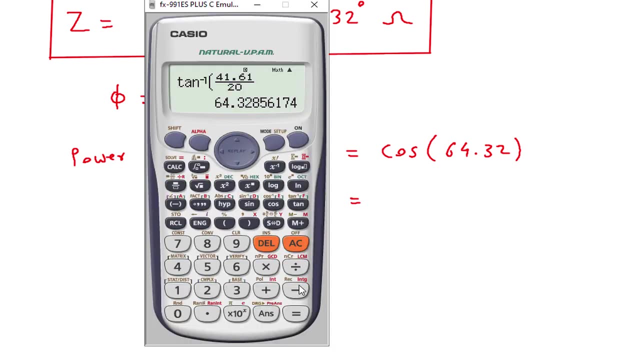 64 .2.. Cos. So this is an element of, And was equal to 64.32.. And was equal to COS and was equal to. The power factor is equal to COP. volt value was 64.32.. So, because this will be a torque of 64.32 in field野. 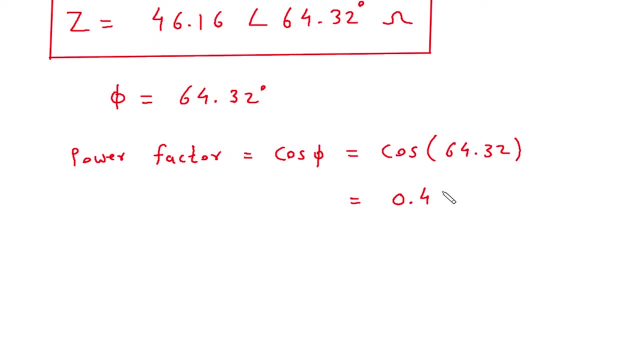 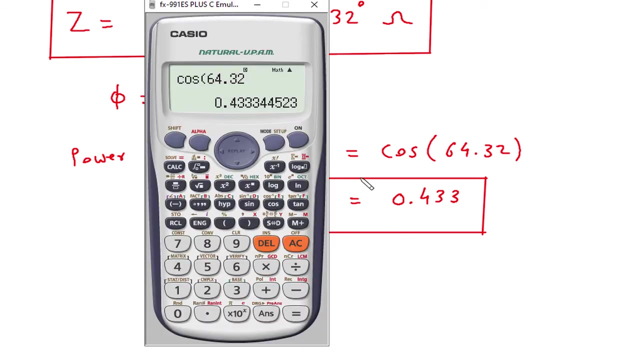 F4. The value is six point two in field, seconds over N, So this will be cos0 point433.. The value is 64.32.. So this will be the value variables. This is the power factor. and power factor have no unit. so it have no unit. and also here we can see: 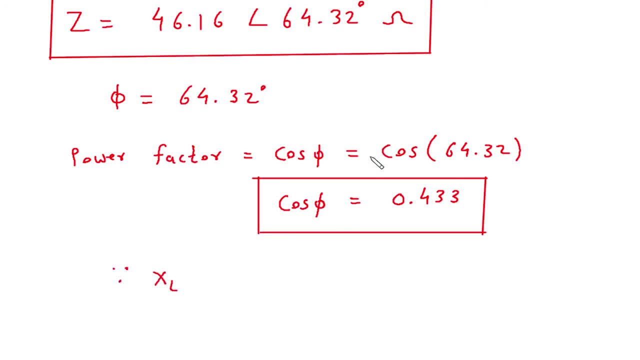 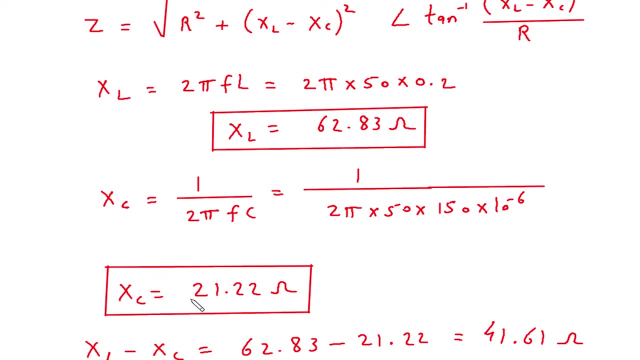 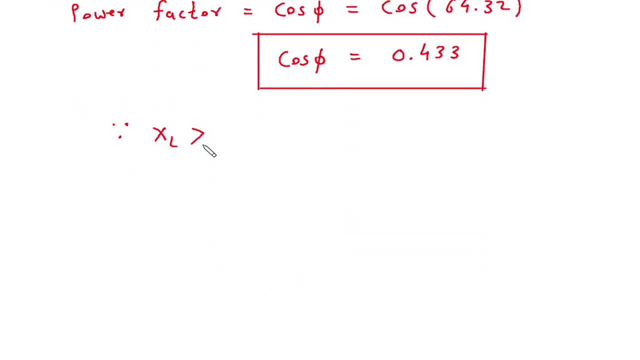 since xl. here we can see the value of xl. the value of xl is 62.83 and the value of xc is 21.22. so xl is greater than xc. so we can write: since xl is greater than xc, so the power factor, the power factor. 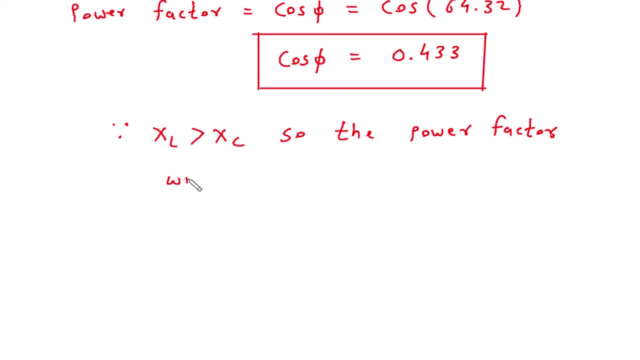 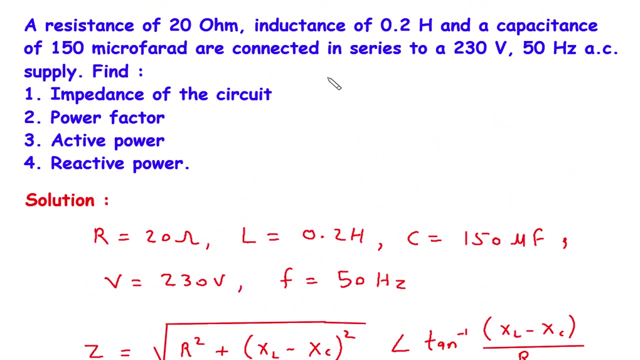 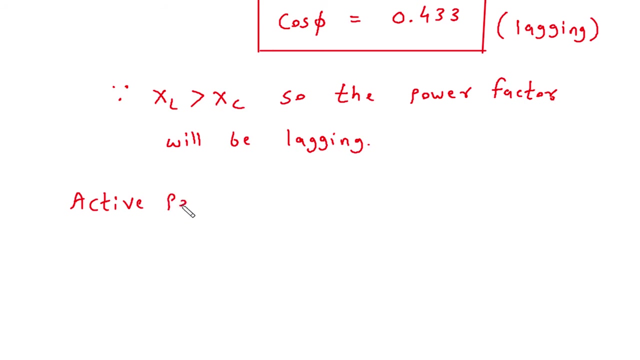 will be lagging. so here the power factor will be lagging. so here the power factor will be lagging. then next we have to find active power, then next we have to find active power. so active power is equal to v into i, into cos, phi. the value of voltage is given, it is 230 volt. 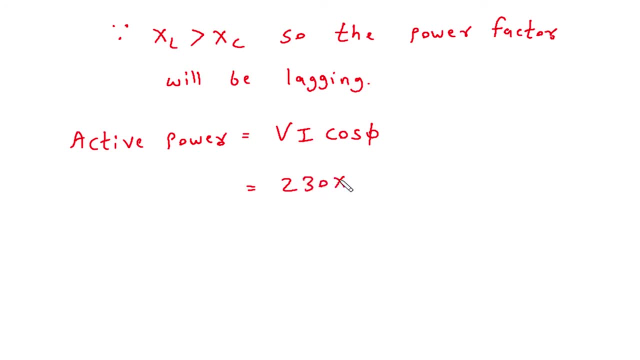 so 230 multiplied by the value of voltage. so 230 multiplied by the value of voltage. so 230 multiplied by the value of current is the value of current is not there. so we can find the value of current using ohm's law for ac circuit, and this will be v by magnitude of z. 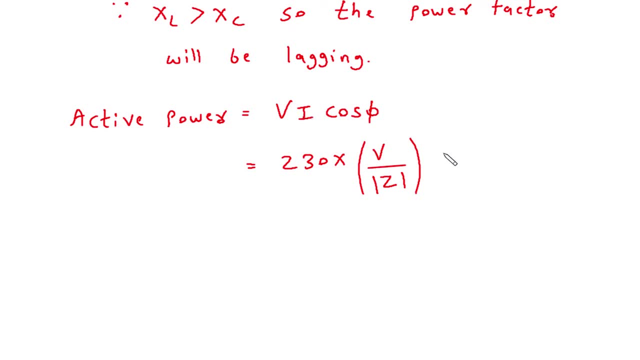 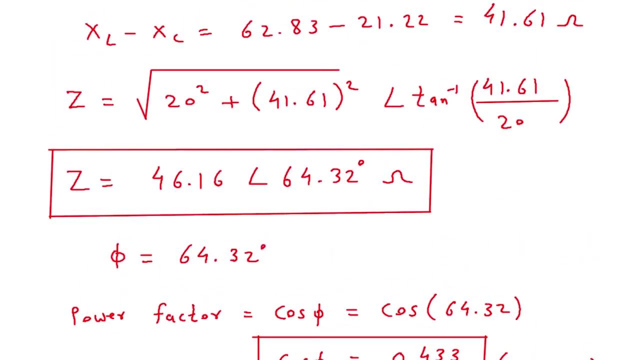 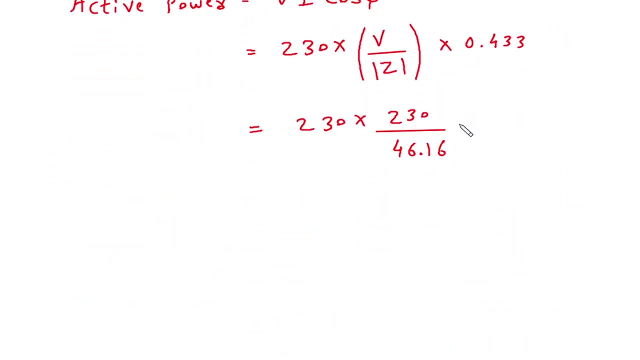 so using this formula we can find the value of this i and the value of cos phi. the value of cos phi is 0.433, 0.433. now we will substitute the value of this voltage again: 230 multiplied by 230 divided by magnitude of z, so mod of z is 46.16, 46.16 multiplied by 0.433. so this will be: